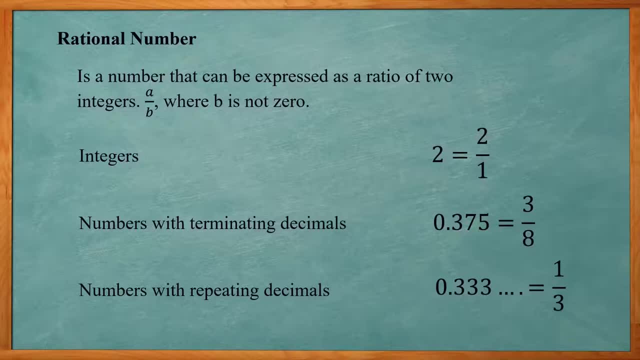 that can be expressed as a ratio of two integers: a over b, where b is not zero. So we're used to integers two. Two can be written as two over one, so a ratio of two numbers, two integers. and then we have numbers that have terminating decimals, like 0.375, and that can be rewritten as: 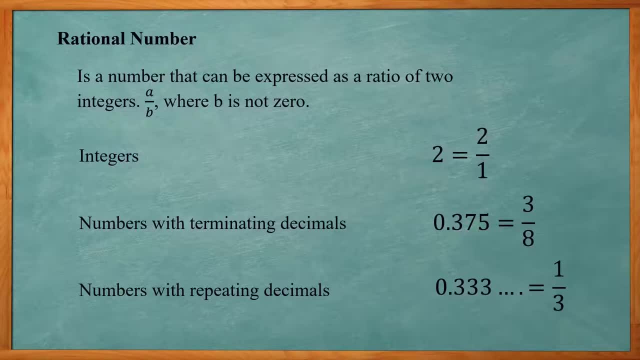 three over eight, so that's a rational number. So a rational number is a number that can be expressed as a rational number. You also got numbers that have repeating decimals. So we have 0.3333 repeating. that can be written as one over three. So 0.3 repeating would be a rational number. 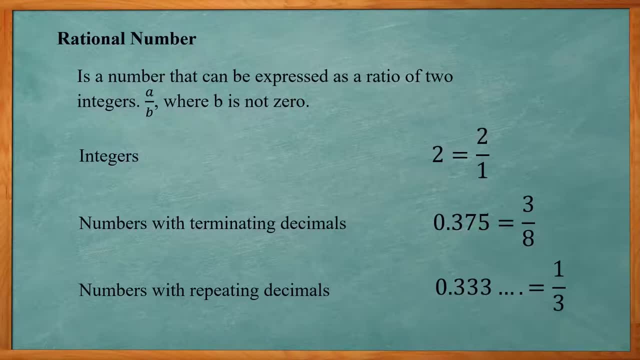 So anytime you have repeating decimals, that's going to be a rational number. If it was all ones repeating, or series of two, five, two, five, if it's some kind of pattern to them, and it can be one, two, three, one, two, three, as long as the pattern repeats, it's a rational number. 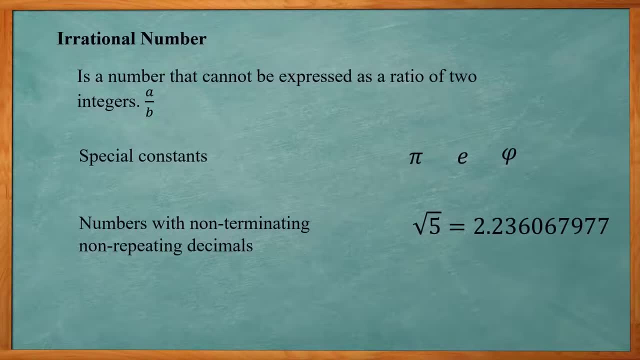 Now for irrational numbers. those are numbers that cannot be expressed as a ratio of two integers, So I can't write it as a over b. You know, some of these include special constants such as pi, euler's number e and the golden ratio, So decimal numbers that are non-repeating and 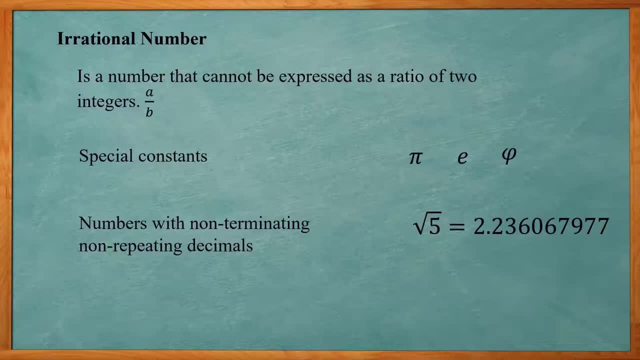 non-terminating are also irrational numbers. irrational numbers: These typically tend to be square roots of numbers, For example the square root of 5, you put that in the calculator, you know it'll show 2.236067977, but this keeps, keeps going and the pattern does not repeat. So 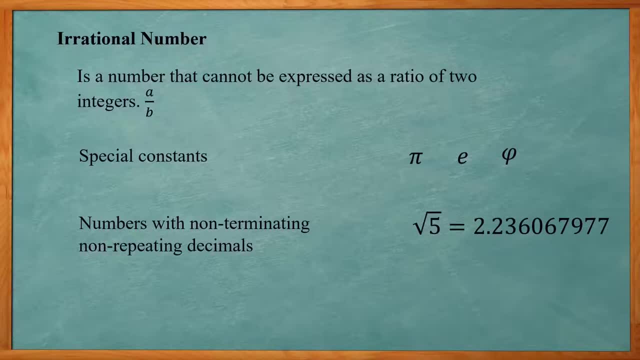 numbers like that- square root of 5, square root of 2, are all irrational numbers. But if I have the square root of 25, square root of 25 is just 5, so that is a rational number. So if it's a perfect square, taking the square root of a perfect 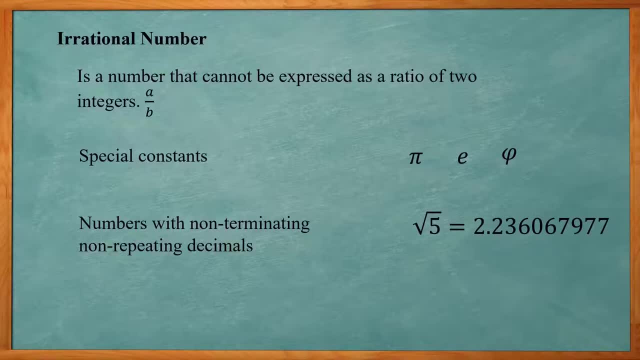 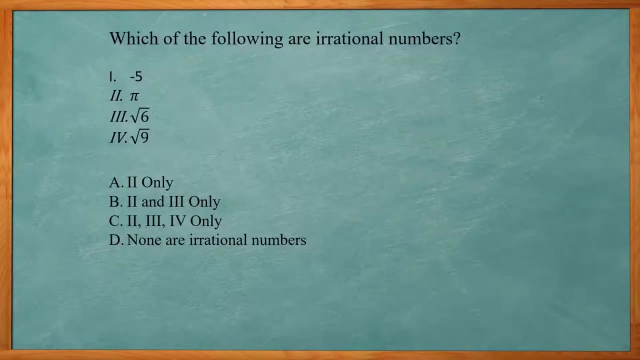 square will be a rational number, But square root of 5,, 7, stuff like that would be irrational. So in this first problem it says which of the following are irrational numbers? We have negative 5,, pi, square root of 6,. 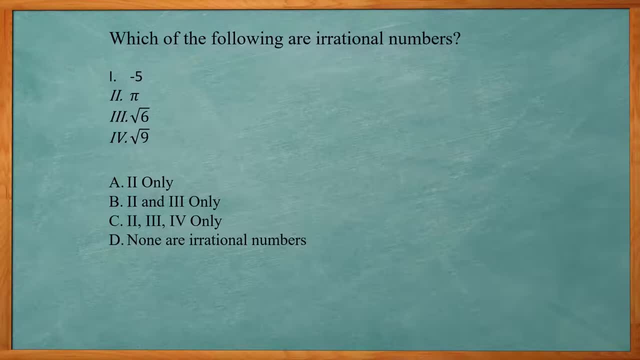 and square root of 9.. So remember, special constants like pi will be irrational. Negative 5 is just a regular integer. it can be written as negative 5 over 1.. Square root of 6 is going to be irrational. it's not a perfect square. 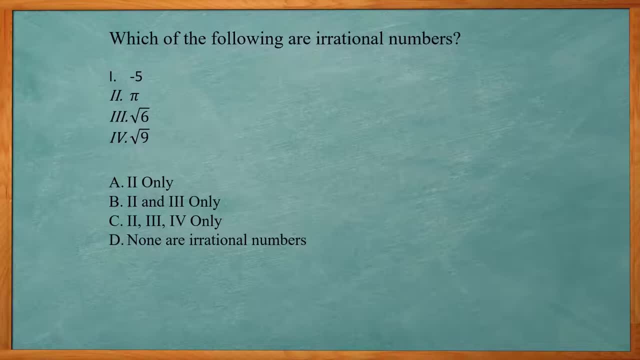 Square root of 9,. 9 is a perfect square, which, so the square root of 9 will be 3.. So it looks like pi and square root of 6 would be irrational numbers. So choice is 2 and 3, letter b will be our answer choice. 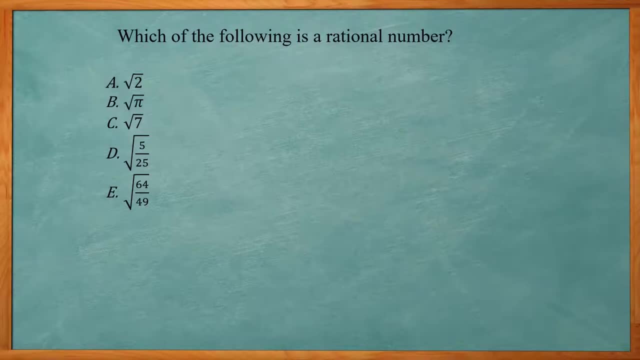 This one says which of the following is a rational number. So remember, a rational number can be expressed as a ratio of two integers, a over b. So we have square root of 2, that's going to be irrational. Square root of pi. we said pi was 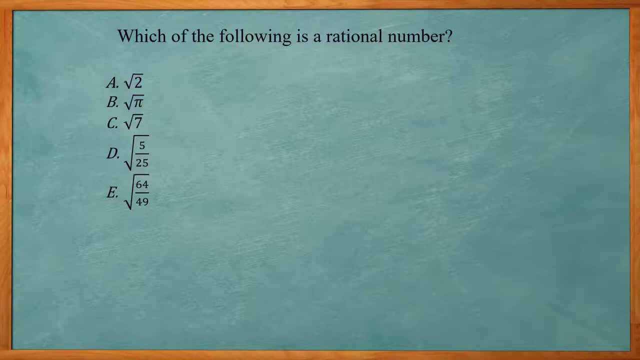 irrational. so the square root of pi would also be irrational. square root of 7,, 8,, 9, and 10.. will be irrational square root of 5 over 25. now remember what square roots. I can rewrite it as square root of 5 or square root of 25, and we know the square root of. 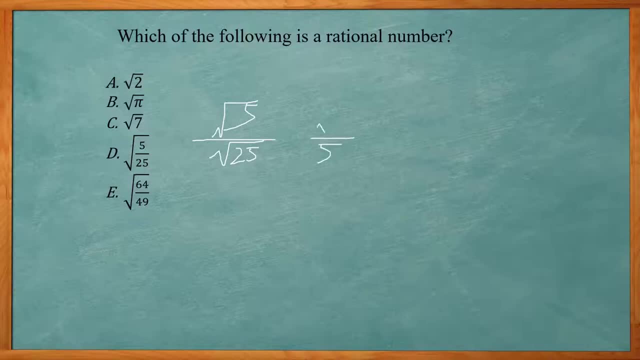 25 is just 5 and then square root of 5 on top. okay, so this is going to be irrational because square root of 5 is now going to be an integer. now, if we look at the last one- square root of 64 over 49- that can be written as square root of 64 over square root of 49. 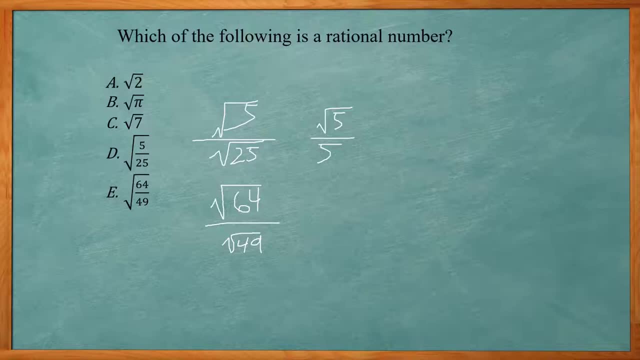 and these are perfect squares. so we have 8 on top and 7 on bottom. so this is going to be a rational number- rational. so this one's asking for a rational number. so another choice: e will be the only one here that's a rational number. 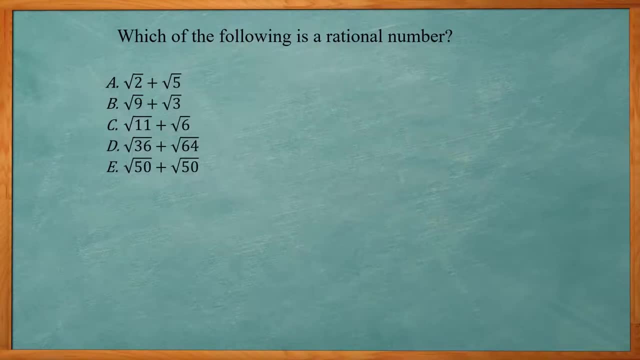 and this one says: which of the following is a rational number? okay, so again we want to look for perfect squares. look at d: square root of 36 is going to be 6. square root of 64 is going to be 8, so that's going to give us a 14 value. all the rest are: